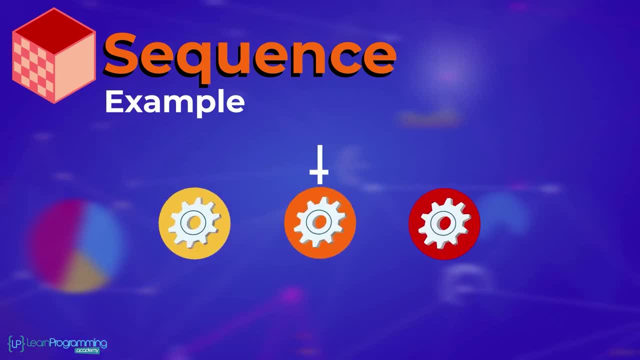 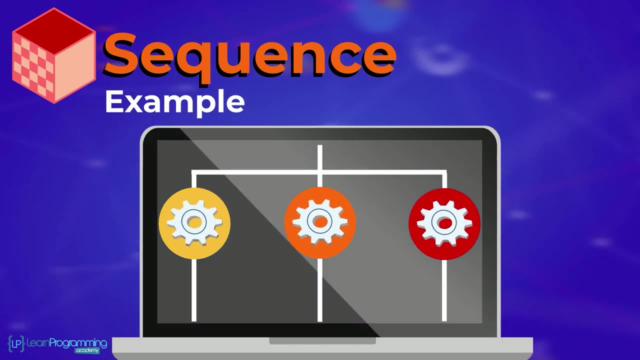 put on your clothes, et cetera. Now, of course, some of these sequential things can be done in tandem or parallel, but so they can be done inside the computer in parallel processing. Now a programming example of this, using English rather than a specific programming language. 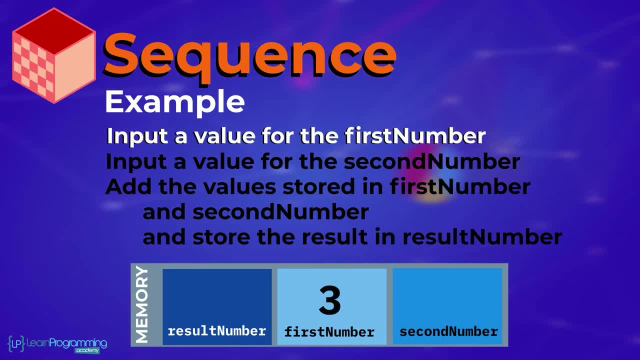 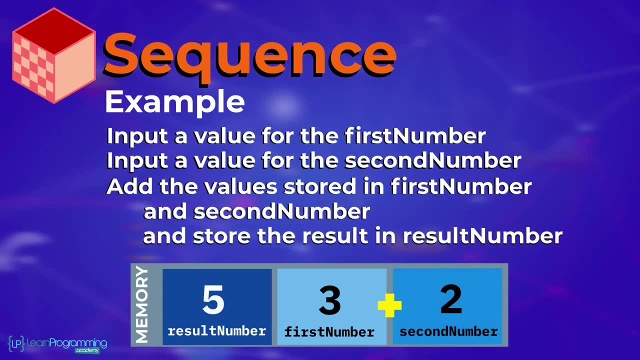 might look like this: Input a value for the first number, input a value for the second number, add the value stored in first number and second number and store the result in result number. The second building block is selection. Now selection in the real world. 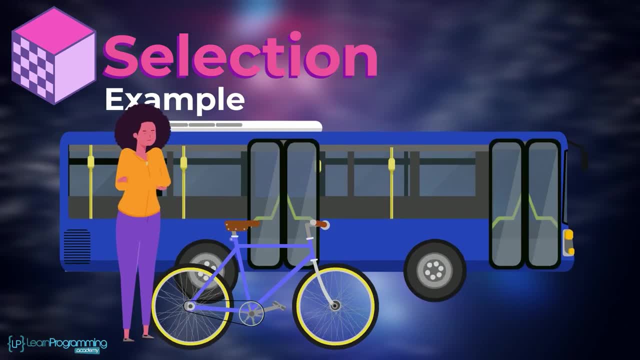 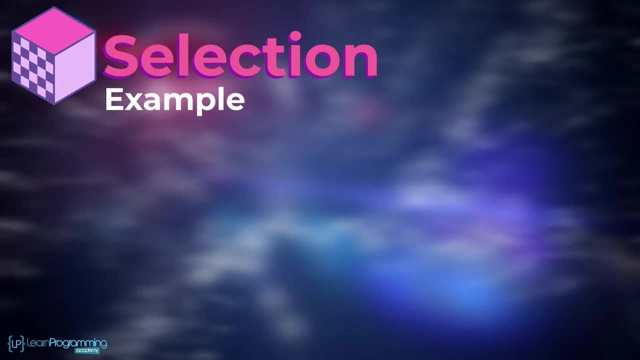 might be you deciding to either ride your bike to work, take the bus to work or walk to work. A programming example of this, using English rather than a specific programming language, might look like this: If the traffic signal equals green, then continue. 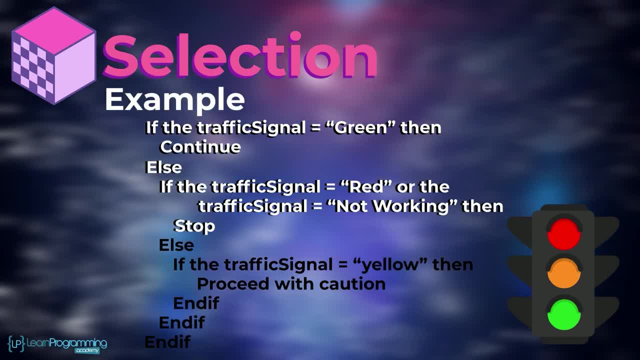 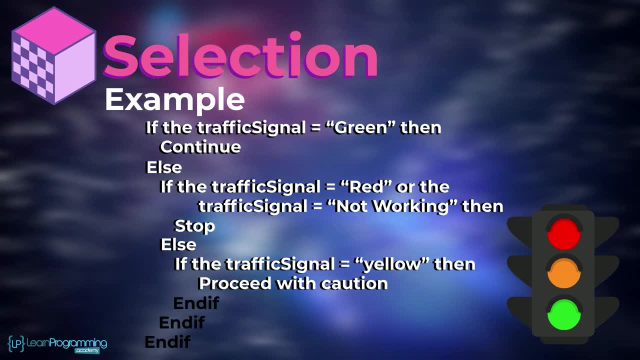 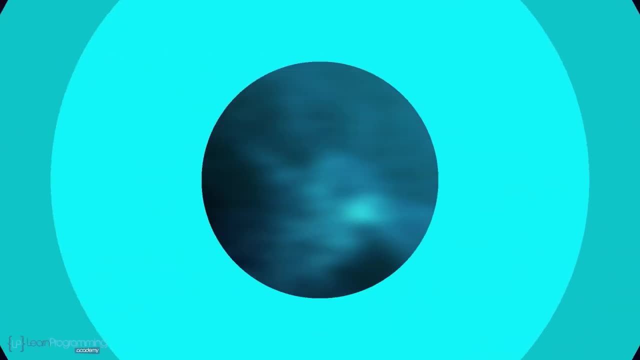 Else. if the traffic signal equals red or the traffic signal is not working, then stop Else. if the traffic signal equals yellow, then proceed with caution. and if and if and if The third building block iteration, also known as looping, 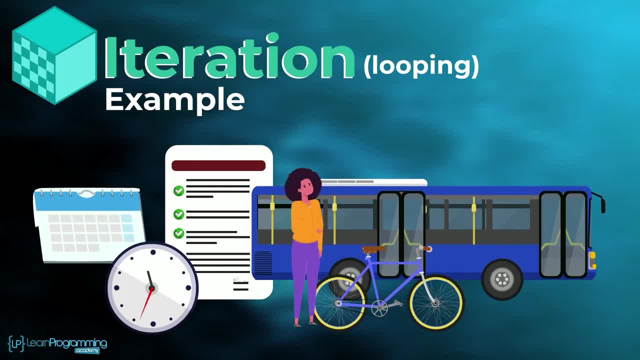 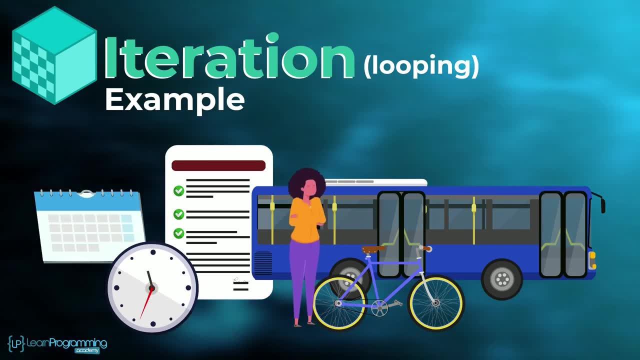 So an iteration, or what we call looping, might be you repeating the same sequence and or selection activities for several days in a row. A very simple programming example of this, using English rather than a specific programming language, might look like this: While I'm hungry, take a bite of my food. 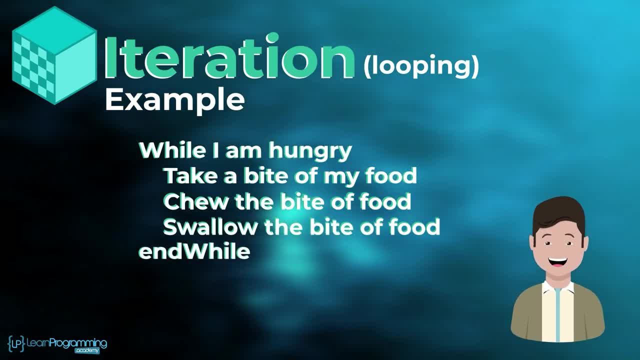 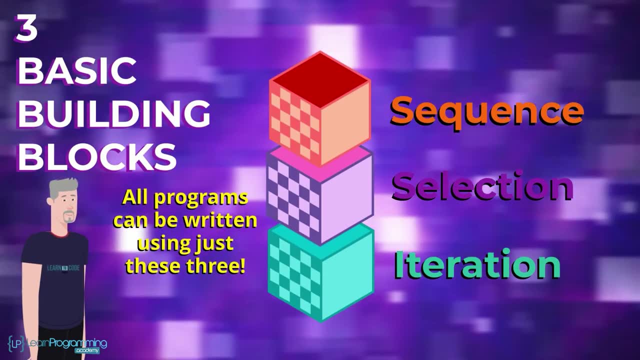 chew the bite of food, swallow the bite of food and while. To summarize, all programs can be written using just these three basic building blocks, and I find that amazing. So just about every computer program contains dozens, hundreds or even thousands or tens of thousands. 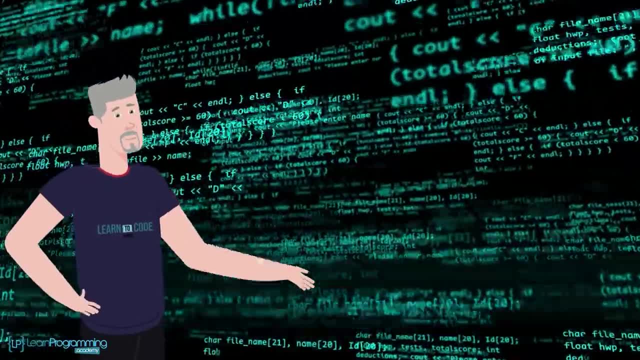 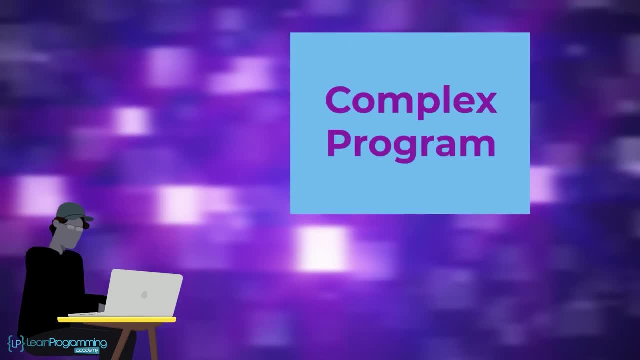 of programming, expressions or statements. I've heard that the Windows 10 operating system consists of over 50 million lines of code. Wow, that's mind-boggling. To deal more effectively with such complexity, programmers break up or chunk their code into smaller parts. 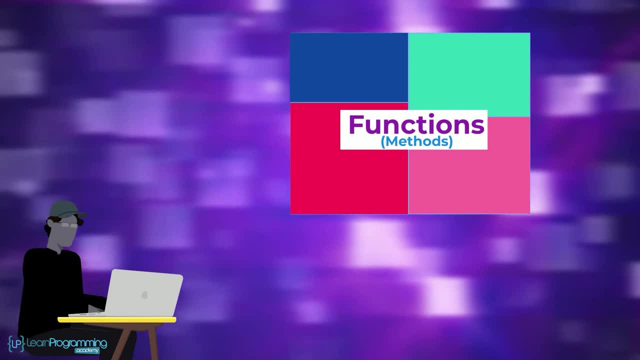 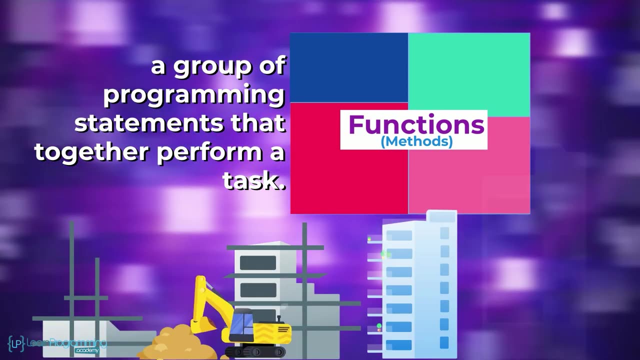 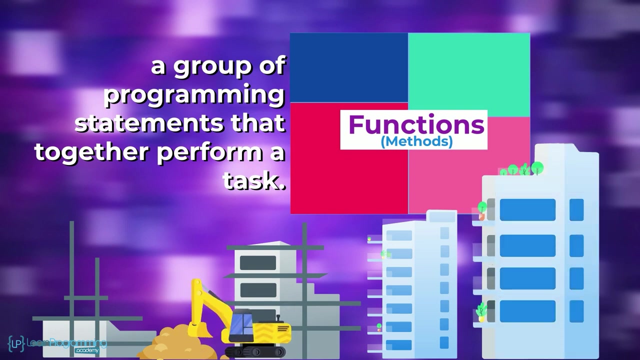 generically referred to as functions or methods. A function is a group of programming statements that together perform a task In the real world. construction projects are always broken up into smaller units or sub-projects to better estimate and perform the overall project. In the software world we do the same type of thing.